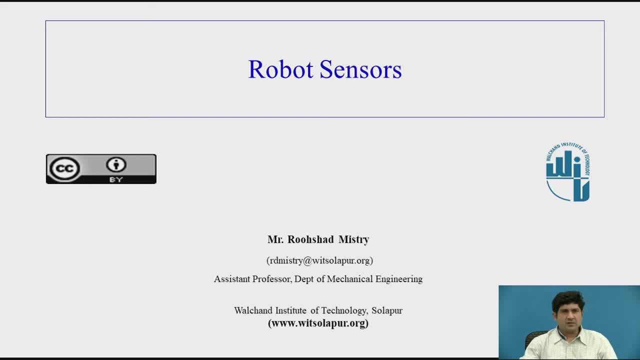 video. So what we are going to do in this particular session is try to look at sensors very specifically from the point of view of industrial robots and, to a certain extent, for mobile robots as well. So the learning outcomes of this particular session are that at the end of the 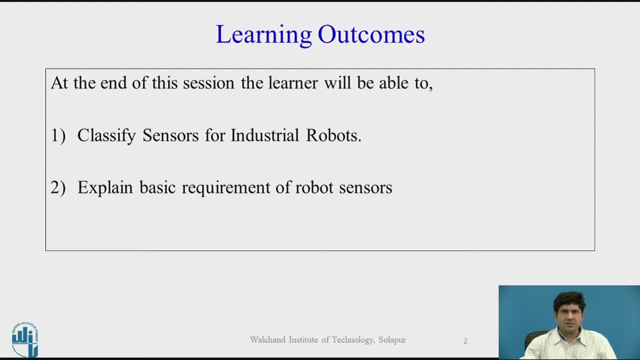 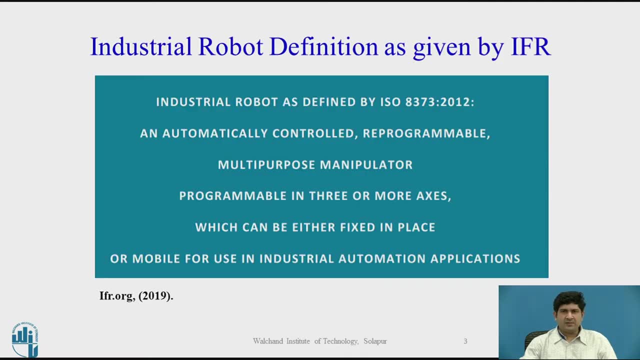 session, the student will be able to classify sensors for industrial robots and explain basic requirements of robot sensors. So before we begin, let us recall the definition of industrial robots as per the International Federation of Robotics, which basically uses the definition given by ISO 8370-2012.. And as per this, the industrial robot is designed to be able to classify sensors for industrial robots and explain basic requirements of robot sensors. So, before we begin, let us recall the definition of industrial robots as per the International Federation of Robotics, which basically uses the definition given by ISO 8370-2012. 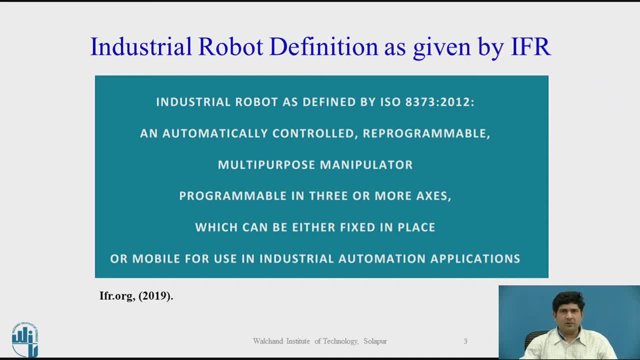 The industrial robot is defined as an automatically controlled, reprogrammable multipurpose manipulator, programmable in three or more axes, which can either be fixed in place or mobile and used for industrial automation application. So I iterate this definition from time to time so that this 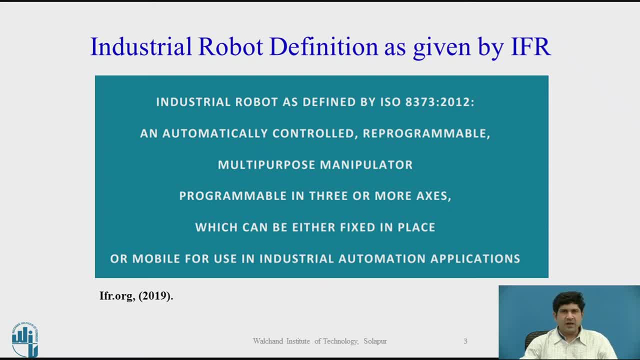 kind of creates a certain consistency when it comes to definitions, And it will also put the context of the sensors that we are going to look at in a minute from the point of view of industrial robots. So let us begin So. the industrial robot is defined as an automatically controlled 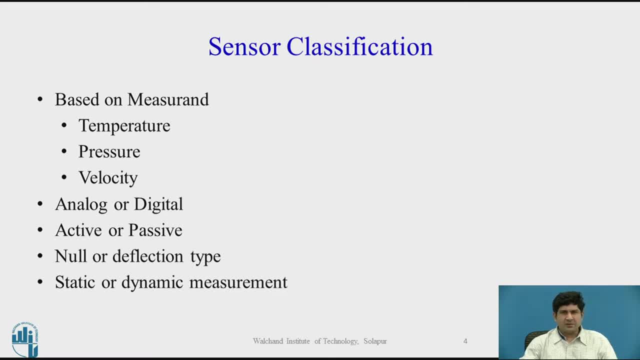 reprogrammable multipurpose manipulator in three or more axes. This is actually sensor classification in general- just a brief review for everyone- And sensor classification. different textbooks tend to have slightly different ways in which they classify sensors. Online sources. 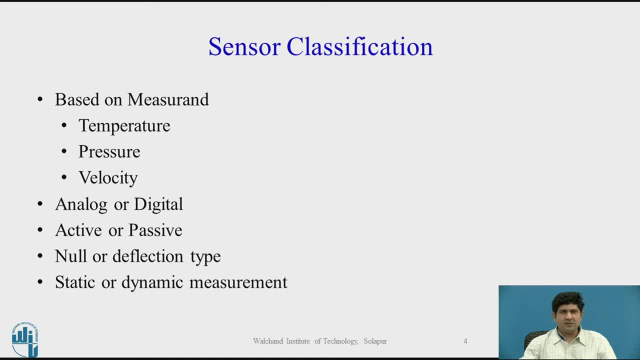 again do the same thing, But by far we can sort of group them into the following categories. So the most common way to in fact classify sensors is based on the measuring. So what's basically measuring? So obviously you have plenty of sensors that you can put under the 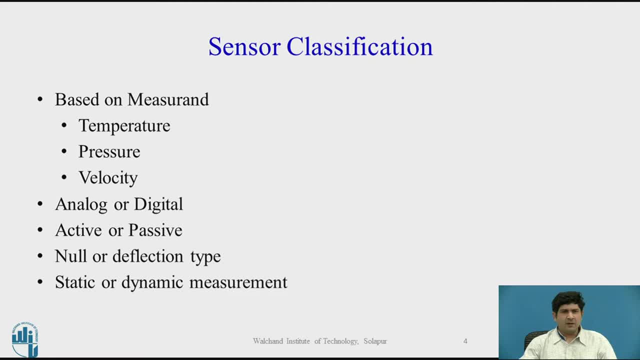 this particular category- temperature, pressure, velocity, flow, any other proximity, and so on and so forth- Then, depending upon whether the output from the sensor is either in analog or digital, you can have a classification of whether you should call the sensor analog or digital. 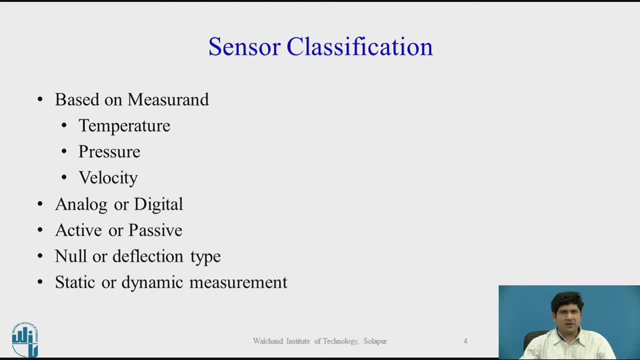 Similarly, based on the source of energy, you can call it either passive or active, And then on the basis of the measurement process, you can call it as a null or deflection type, And then again whether the sensor measures a static or a quasi-static parameter. 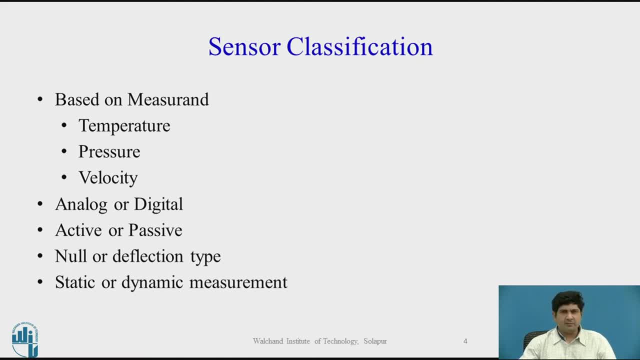 whether it's meant for dynamic measurements such as vibration. you can classify them accordingly. Now, a very good book, if you want to refer to sensors, is Measurement System by Dieblin. There are plenty of other books, for example Instrumentation Handbook. 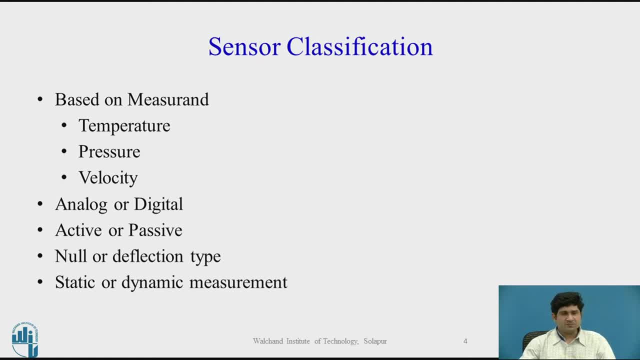 And I definitely encourage you to read these books if you want to get more information regarding sensors, how they are classified, characteristics and so forth, And we have covered some of this portion, definitely in some of the previous lectures. Now, when we look at 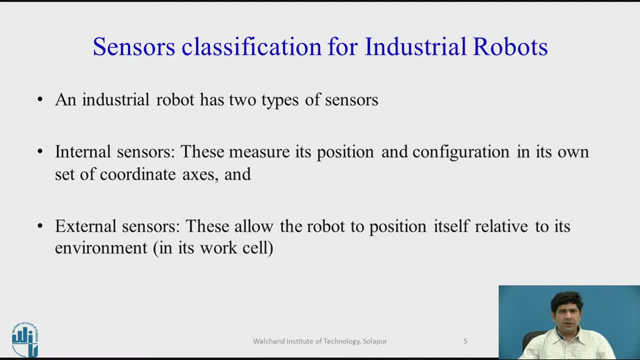 robot sensors in particular, and this is not just for industrial robots. I have seen a similar kind of classification for mobile robots as well, And even textbooks tend to agree on this particular direction. So industrial robot sensors: typically we classify them as internal or external. 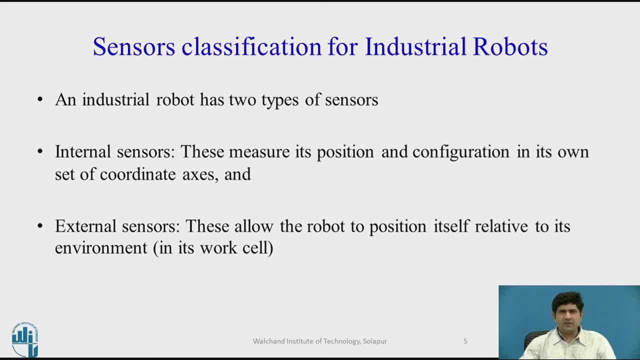 So, remember, all industrial robots have server-controlled joints and there is a need to know what the correct position of the joint is, what its velocity is and how the robot is positioned in that position. And for this we have encoders And the best. 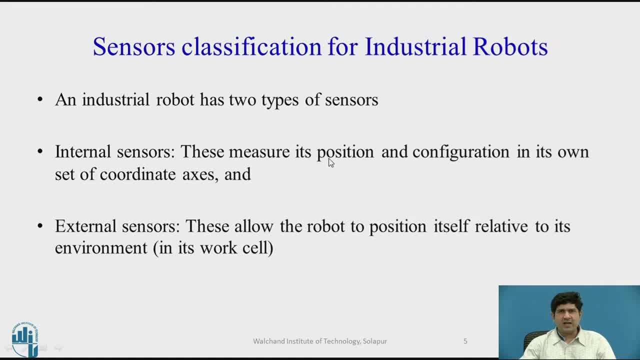 example that we can give for these. internal sensors are encoders, So these measure the position and the configuration in its own set of coordinate axes. Therefore we call them internal. They give an estimate regarding the internal state of the sensor. External sensors, on the other hand, 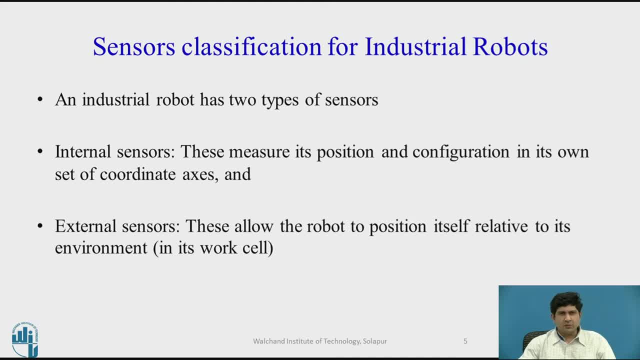 allow the robot to position itself relative to its environment, that is, within its work cell. So these include, to a certain extent, proximity sensors, force sensors, visual sensors and so on, And these include the exact coordinates of the robot in its own set of coordinates. 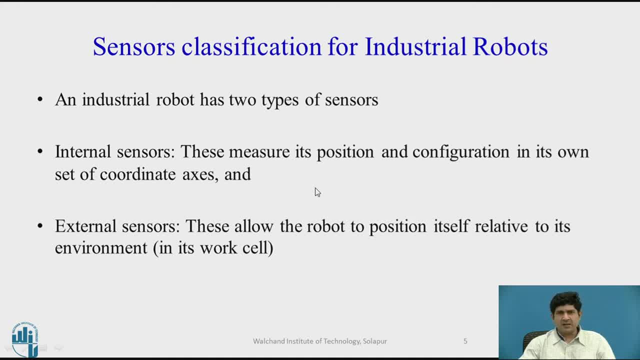 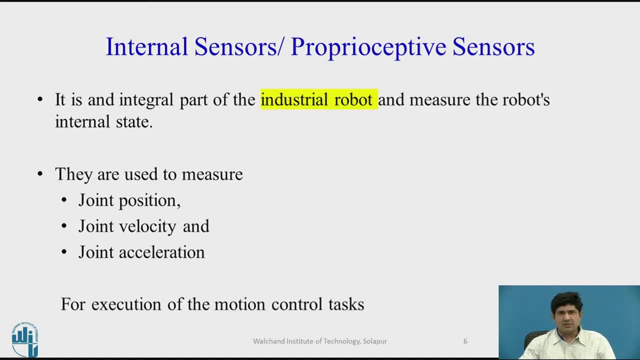 vision systems that will typically fall under this category. So let us look at these sensors into slightly more detail Now. internal sensors, also sometimes called as proprioceptive sensors. So these are integral part of the robot and, like I said, they measure the robot's internal. 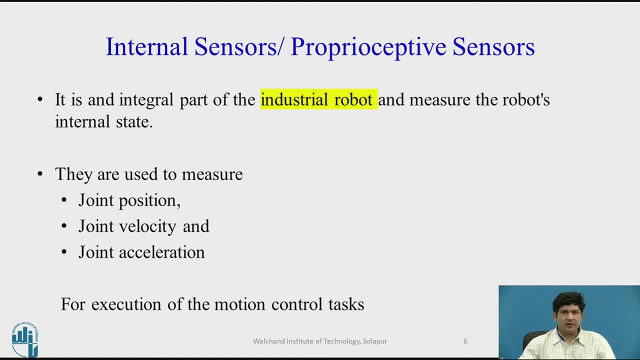 state and these are typically the ones who measure the joint position, the joint velocity and joint acceleration in case of industrial robots, and these are absolutely essential for the execution of all motion control tasks. So basically all the control algorithms which are joints, position servers, velocity servers. 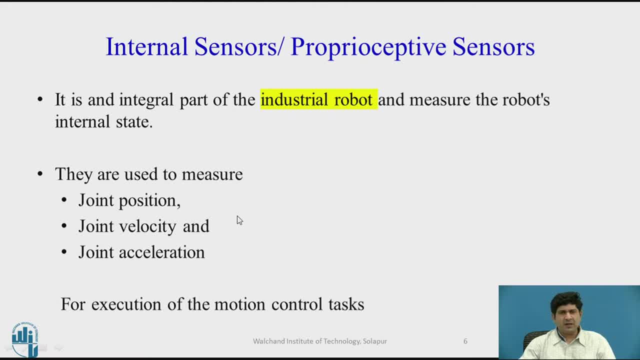 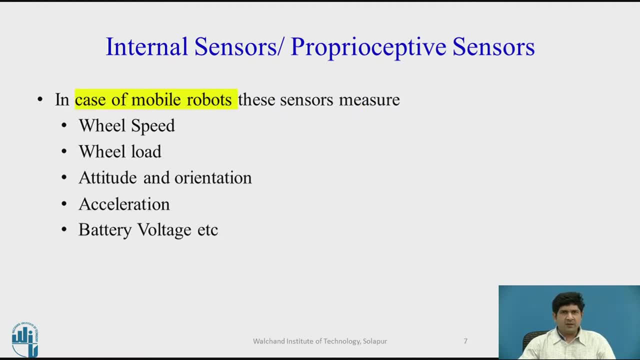 and acceleration control systems. they will all depend upon the feedback given by these sensors in order to execute the control task. The next case, in fact, when we look for mobile robots. I have included this particular paragraph over here because there is quite a bit of write up available on mobile robot sensors. 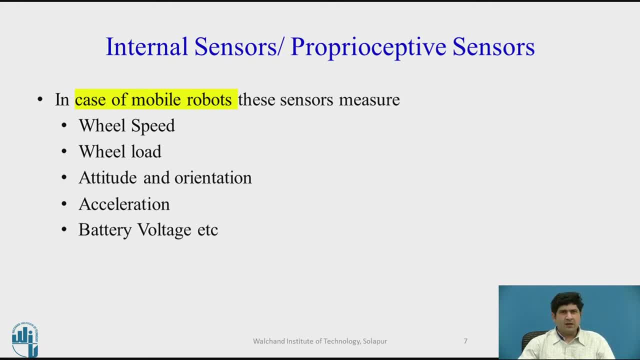 as well online. So if you take a look at mobile robots Now, though, in a very classic sense, lot of books will not include mobile robots under the heading industrial robots, in which we mainly actually study manipulators, but it was prudent, given the proliferation which is happening for mobile robots, to include 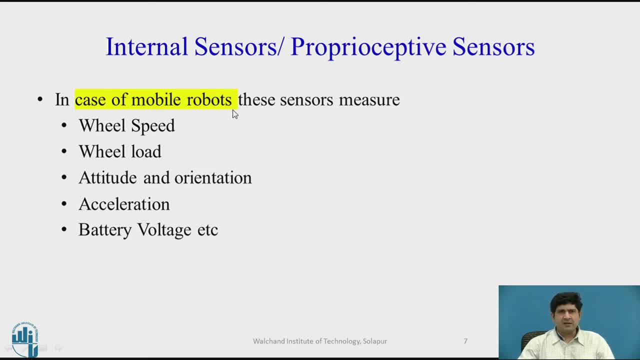 these as well, and in case of mobile robots, typically we can classify internal sensors as wheel speed sensors. we have wheel load sensors, the attitude and orientation, acceleration and battery voltage, So they give an idea regarding what is the state of the mobile robot. 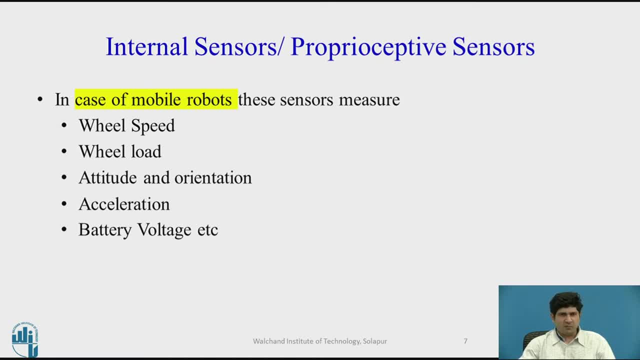 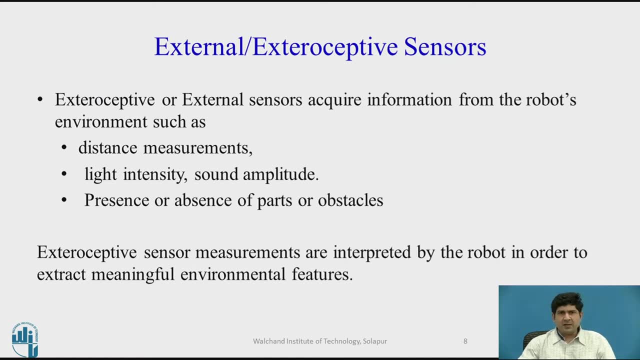 I have mentioned a few. in fact, there may be a couple of more which you can add to this particular list. So coming back to it now, external or exteroceptive sensors: these acquire information from the robots environment and these are basically even for distance measurement. they do light. 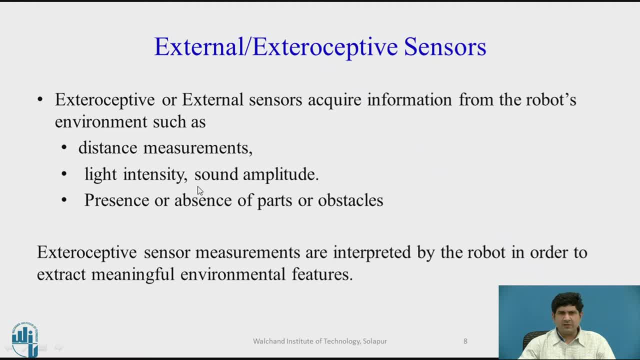 intensity calculation or so on, but they give an estimate where the robot is in its environment, in its work cell. So the sensor measurements are interpreted by the robot in order to extract meaningful environmental features. Now this is especially in the case of, let's say, tactile and force sensing, where it tries 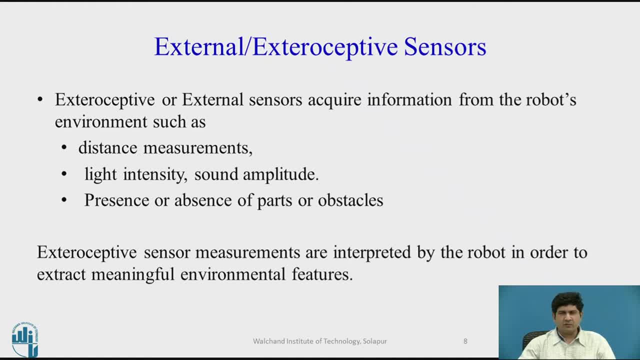 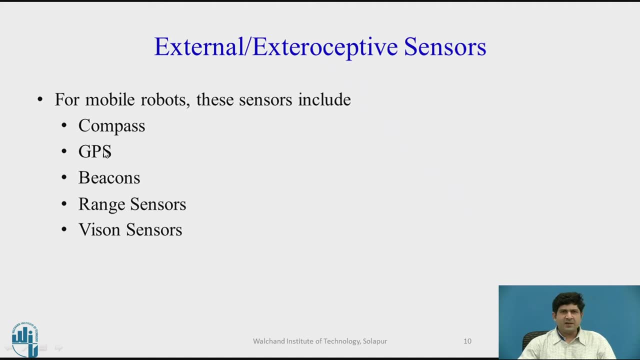 to estimate presence or absence of a part, and so on and so forth. Vision system, obviously, is also an external sensor in this particular case. Now, when it comes to mobile robots, again external sensors are a compass: GPS beacons, rain sensors and vision sensors. 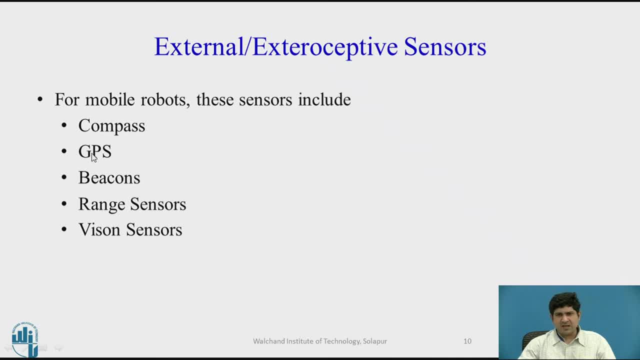 Now, when it comes to GPS global positioning systems, I have come across a couple of resources who have included them under internal sensors, but I have decided to include them under external over here, because they give a position of the robot in the environment. So they are. it doesn't give the state of the robot in itself, but where it is located. 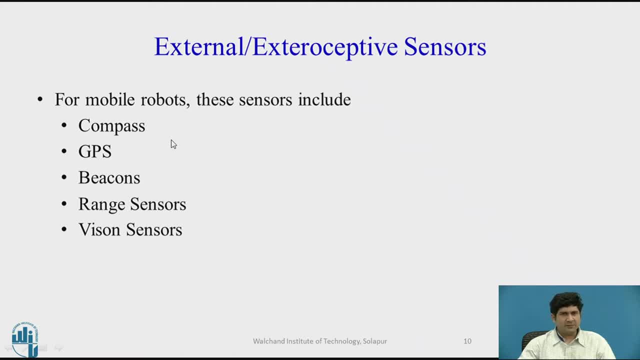 So that's why it's more prudent, in fact, to put them under this particular category. Vision sensors, for example, mobile robots use for navigation, So they have a lot of information For ranging for obstacle detection and so on and so forth. So, again, there may be plenty of sensors you may add to the list, depending upon what the 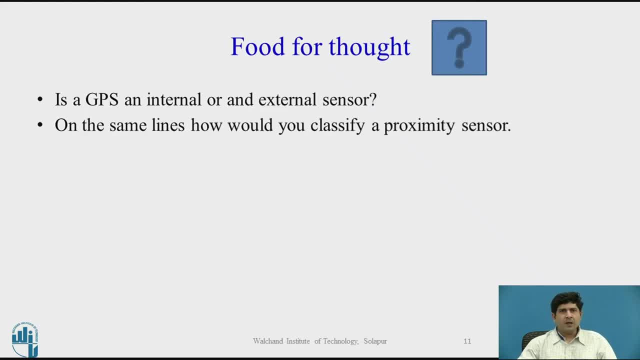 features of the robot are. So that's why something for you to think about is GPS and internal and external sensor, and, on the same lines, how would you classify a proximity sensor? The reason I have this discussion is sometimes you may come across Sources which tend to contradict a few things. 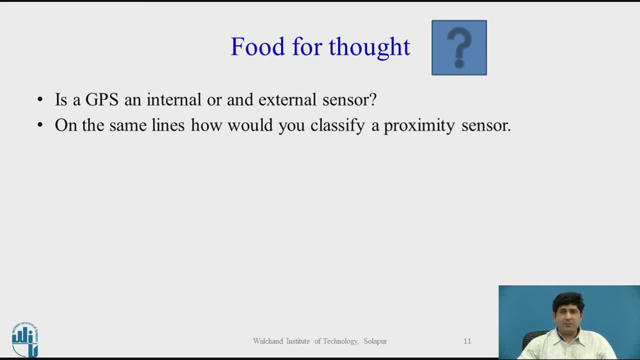 And I have seen this in the past- in both senses sources appear to be quite credible in the sense they are from reputed universities, And this often creates confusion among students. So sometimes I keep this discussion open so that we can draw some conclusion from the various sources that we come across. 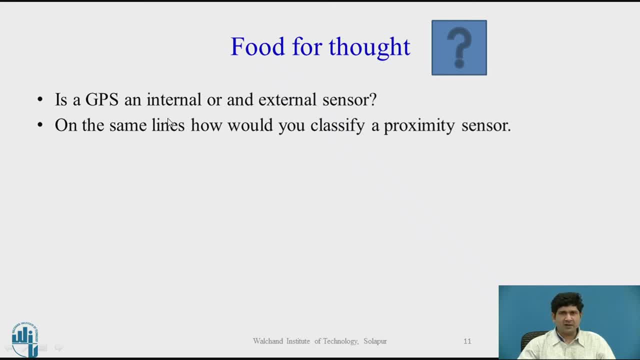 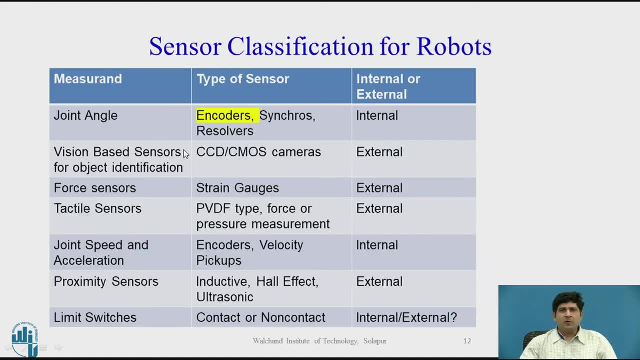 And let's- I'll also try to find out in what context that particular author has gone ahead with his way of talking. So let's look at some of the sensors that we can use to classify a proximity sensor. So once again here, I present you a table of different sensors that you typically find. 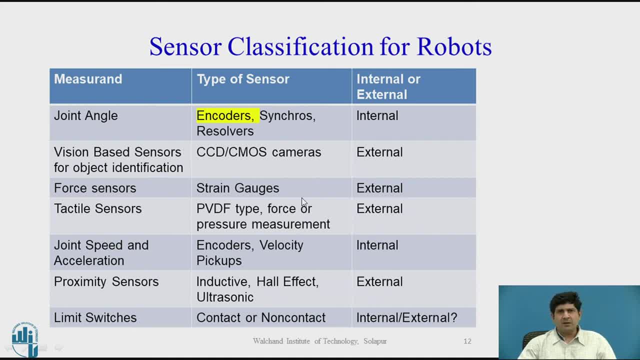 in robots And whether you should classify them as internal or external. So, typically, if you're measuring joint angle, the types of sensors you use are encoders, synchroners, resolvers, encoders being by far the most popular optical encoders which 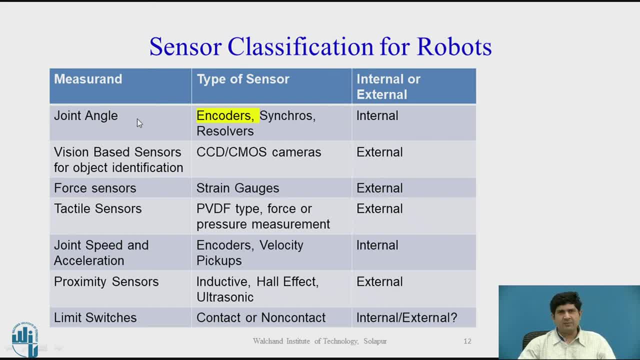 use gray code. Very popular, Very popular sensors when it comes to joint angle measurement. Obviously these are internal sensors. Then you have vision based sensors over here for object identification, And typical sensor is either a CCD or CMOS camera. Nowadays CMOS is gaining popularity, though in machine vision applications CCDs still. 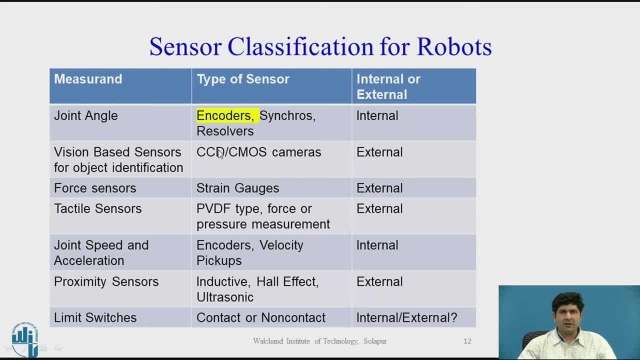 have the majority of the market share, But if you take a look at your mobile and handheld devices, then in that case CMOS cameras typically rule the market. These are obviously external sensors. Then you have visual sensors, Then you have force sensors, which basically measure the force that the robot is executing. 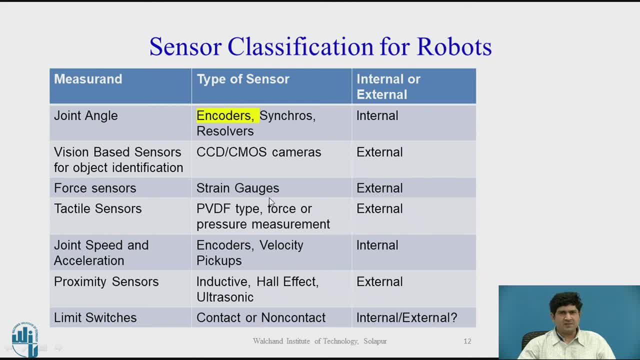 in order to complete a task And strain gears are by far the most popular sensors for this. These are again obviously being external sensors. Similarly, you have textile sensors, which can be of different types. These are also external sensors. Then you have joint speed and acceleration. 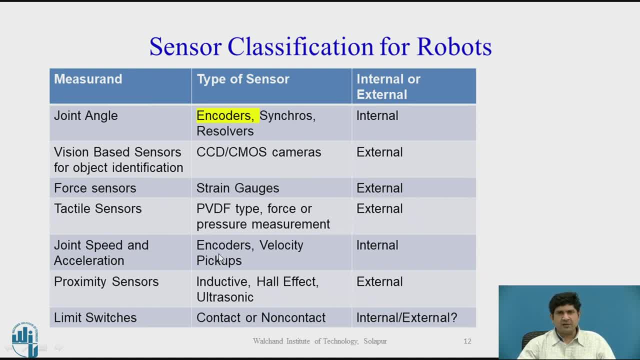 This is necessary for the robot to execute a certain trajectory and hence these are internal sensors. So you can see here, in many cases the encoder signal in fact is differentiated to get velocity and which is again differentiated to get acceleration. But there may be tachometers and pickups which may be specifically meant for velocity measurement. 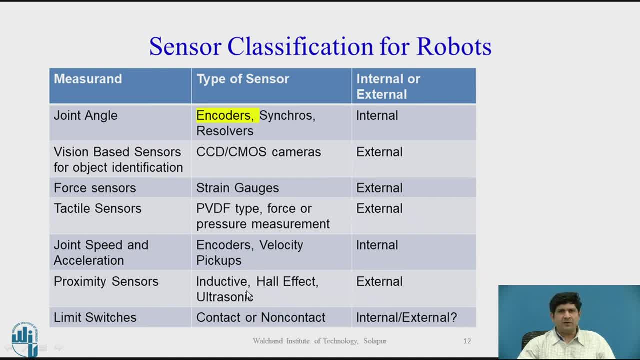 as well. Then you have proximity sensors, which may be inductive, Hall effect, ultrasonic and others, And these are again external sensors. Now the interesting part is limit switches. So these are contact or no contact type. Again, I have read a couple of resources in which they have given up. 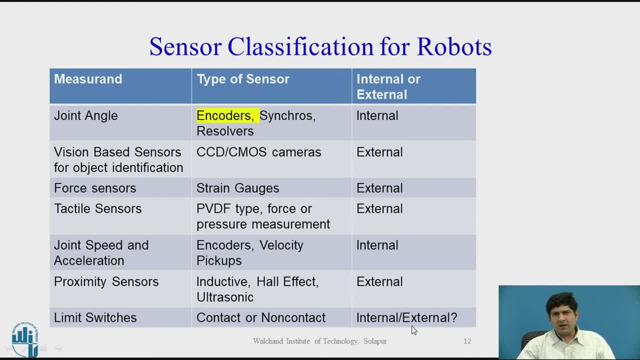 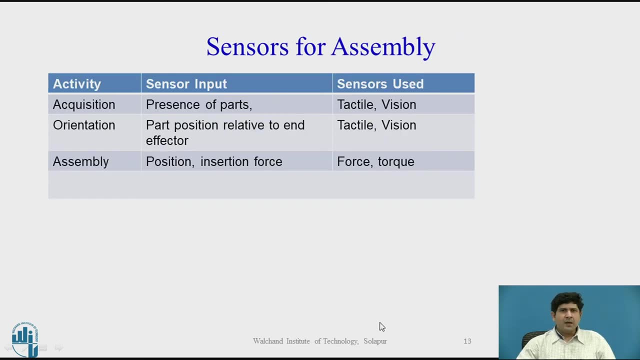 Alternating definitions for these, But I prefer to put them as an external sensor rather than an internal sensor, Because it is not meant really for a feedback, but it is sort of a protection aspect. so it is better grouped in as an external sensor. Now, when it comes to sensors for a specific assembly task, just to put things into context. 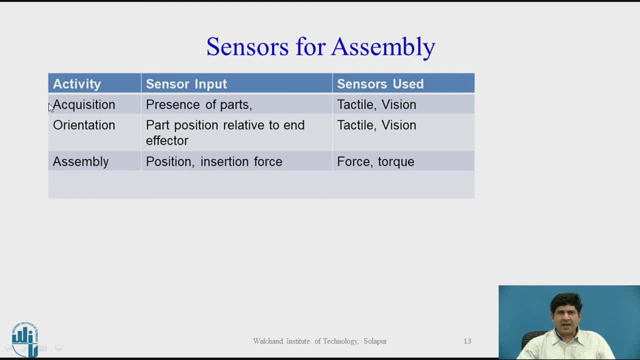 I have included this. If you are doing acquisition, What we need is we need to understand the presence or absence of parts, And typically the sensors that will be used here will be tactile and vision sensors. Similarly, if you want to orient it, that is, you want to orient the robot or the part relative- 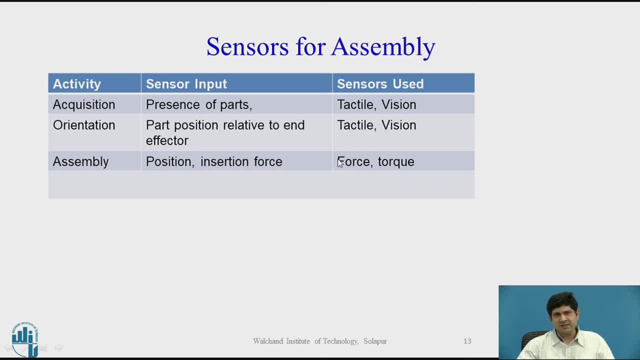 to the end effector. In this case, again, we need tactile and vision sensors, And then for the actual assembly process we need the position and the insertion force, for which we need force and torque sensors, along with some active or passive compliance devices. So, just to put things into context, I have included this particular team. 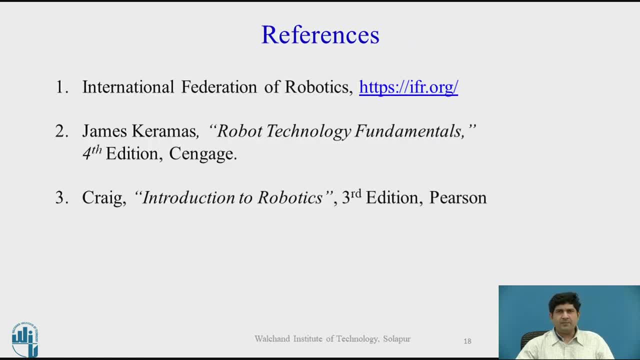 There are plenty of information available for this online. I recommend the textbook James Karamas, which gives you a good overview for what sensors are. In addition to these textbooks, I definitely encourage you to visit the robot manufacturers themselves. They have a very interesting product line up from which you will find very pertinent.